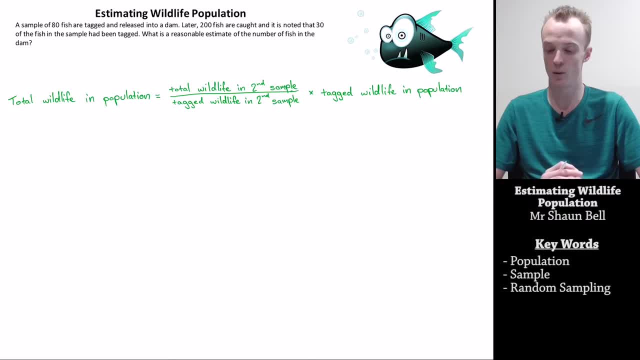 released into a dare. Later, 200 fish are caught and it is noted that of the 200 fish, 30 of them in the sample have been already tagged. What is a reasonable estimate of the number of fish in the dare? So when we're using our formula, we first need to work out what is the total wildlife. 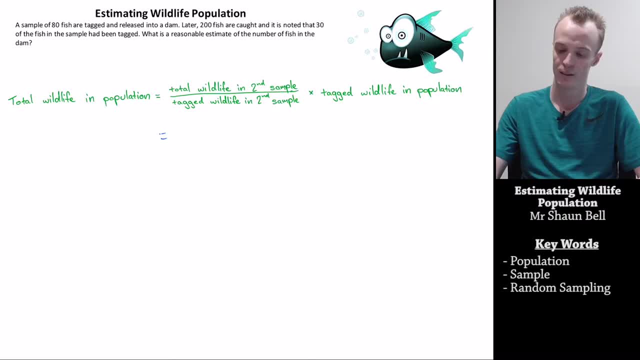 in the second sample. So if we highlight it here, the second sample has 200 fish. So therefore 200 is on top of the fraction here. On the bottom of it we've got tagged wildlife in the second sample. If we looked at how many were tagged in the second sample, we note that 30 of the fish 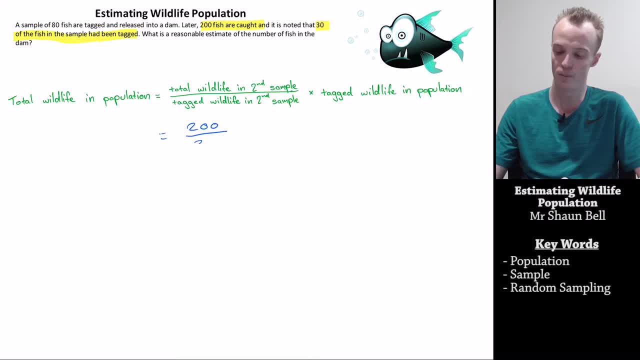 had been tagged. So on the bottom of our fraction it's going to be 30. Then we multiply this with the tagged wildlife in population. Now the total tagged wildlife in population came from the first sample that we tagged. We tagged all of the first sample. 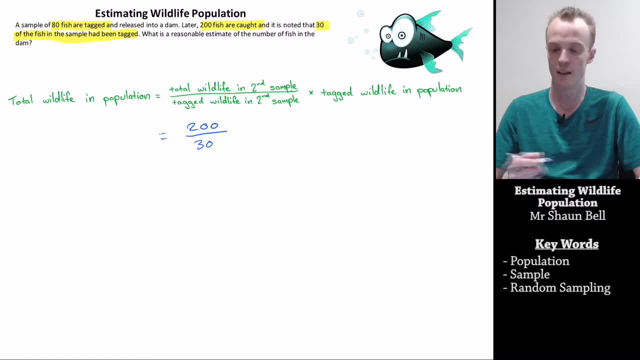 And the first sample had 80 fish that were tagged. So therefore we multiply it by the 80 fish that were tagged. Now, when we multiply this out, we find that the total number of fish in the second sample is approximately 533, and one-third fish in the damp. 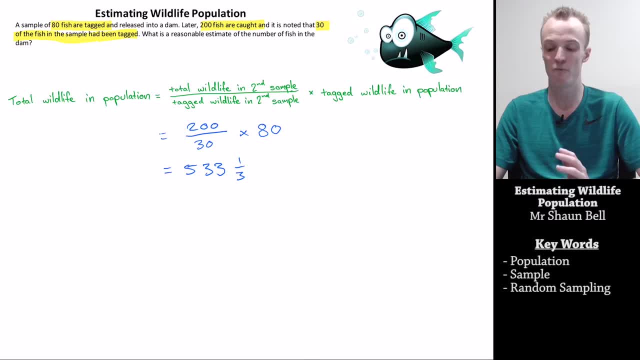 However, this is only an estimate And we've been asked to provide a reasonable estimate. Now what that means is we need to interpret this. A reasonable estimate would probably be to the nearest 100 in this problem. So therefore, there is approximately 500 fish in the damp. 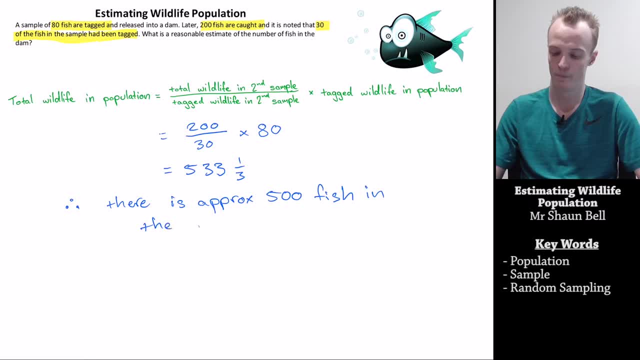 Okay. So to recap, in order to provide an estimate of the wildlife population, you first need to capture, tag and then release a sample of the population. Then you catch a second sample of the population and you need to look at how much of that population. 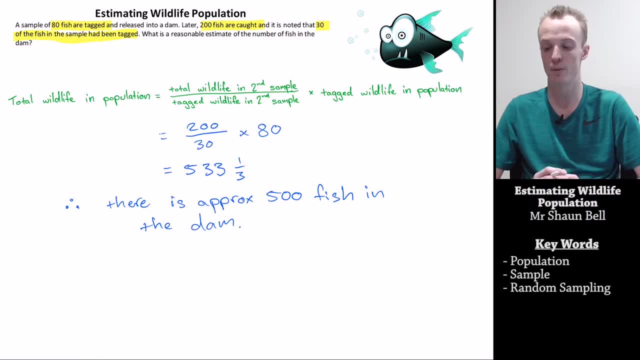 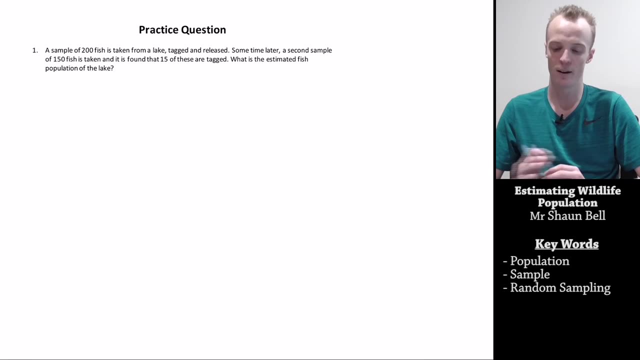 is tagged. how big was the second sample? and you take the second sample, divide it by how much was tagged And then multiply it by how big your first sample was. So now let's have a look at a question for yourself.